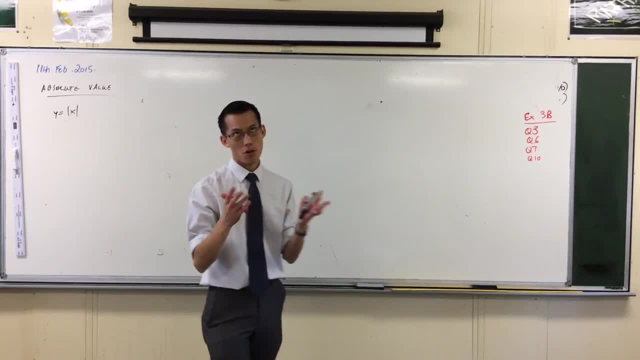 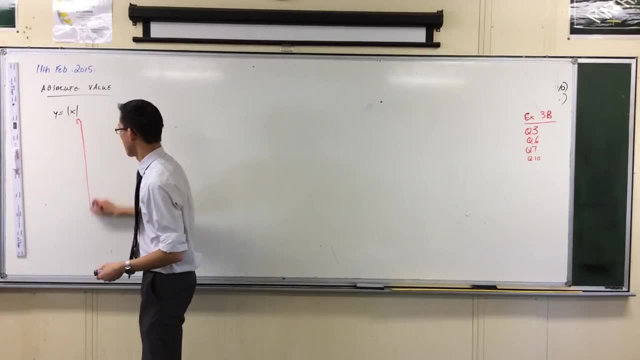 Now you can think about this two ways- Well, more than two ways, but at least two ways, based on the definitions that I gave you the first time. I talked about absolute value, So example: First way you can think about it is just take the positive value. 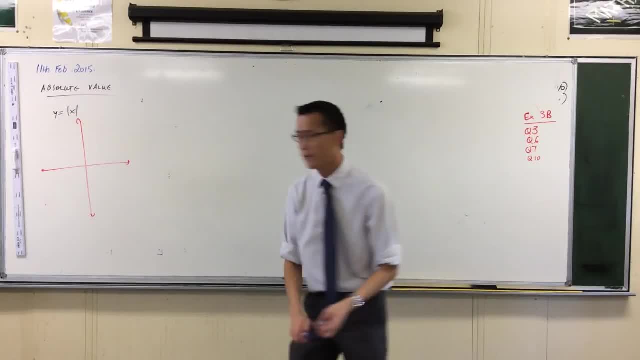 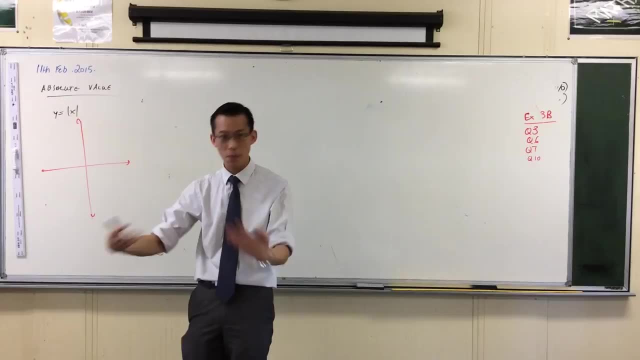 That was the most basic definition I gave you. So therefore, you say: well, this is like y equals x, and I know what that looks like. but you just take the positive values. So here's y equals x. There you go, Good old y equals x. 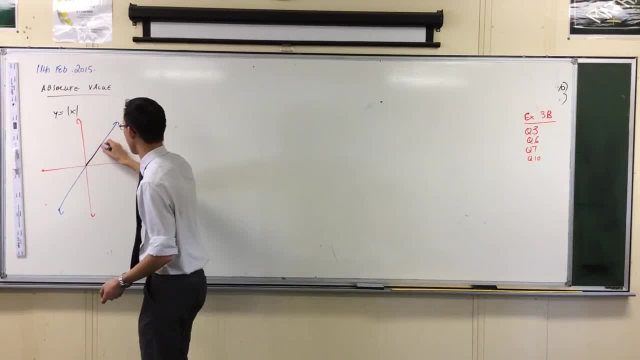 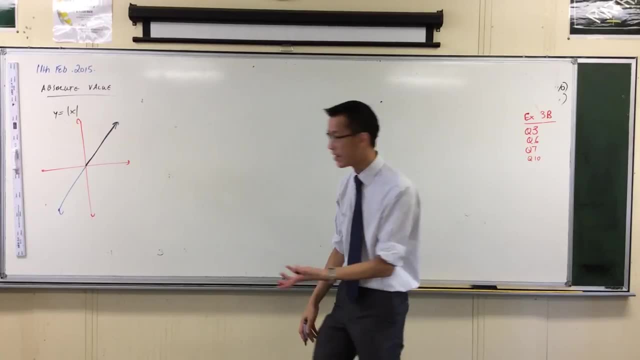 Some of it is positive, so no problems, There you go. That part's all happy times. But on the left-hand side I have a whole portion of the graph that is negative Right, So instead I make that part positive. 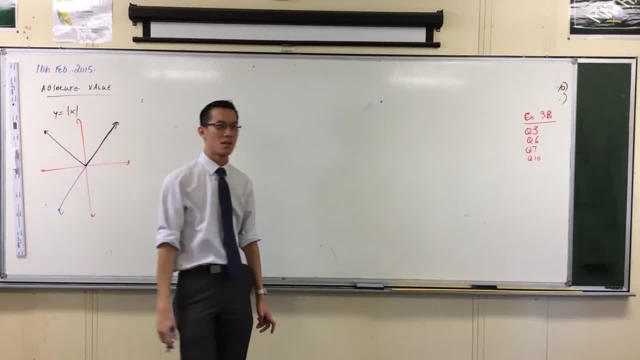 Right. So most people learn about absolute value graphs as: oh yes, the bouncy things. Right, Because they come down to the axis and then they literally bounce. Okay, That's not that complicated. Let's think about a couple of variations on this. 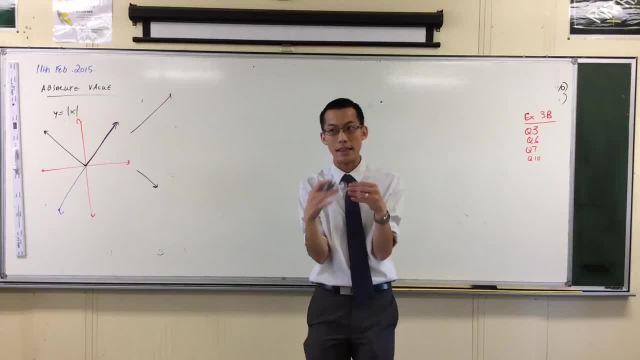 Let's think about: First, let's modify something. it within the absolute value sign. so if I said, well, how would this thing be different? okay, so we've looked at this before. briefly again, I'm going to go to this idea of thinking about: what does X minus 1 look like? okay, and it's just. 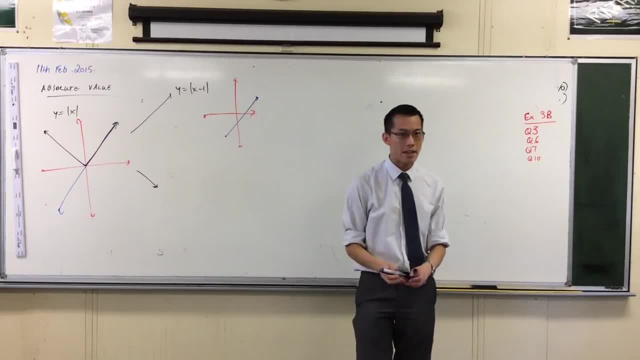 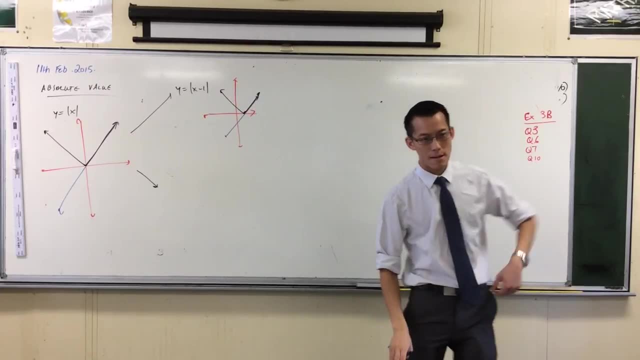 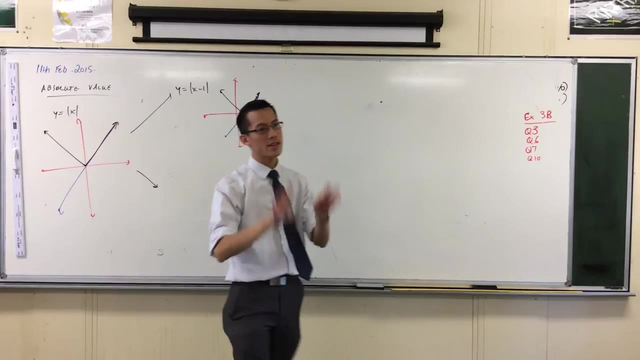 like X, but drop down right, and then again I think, well, I just want the positive parts, so this bits good and this bit is not okay. now this is a really important point under absolute value graphs. I'm going to put this on both of them, because what you've got is two branches that are behaving. 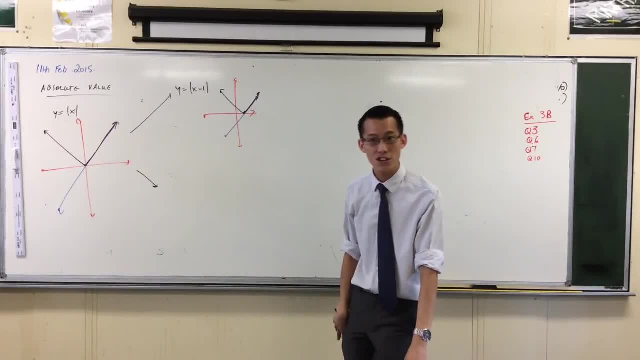 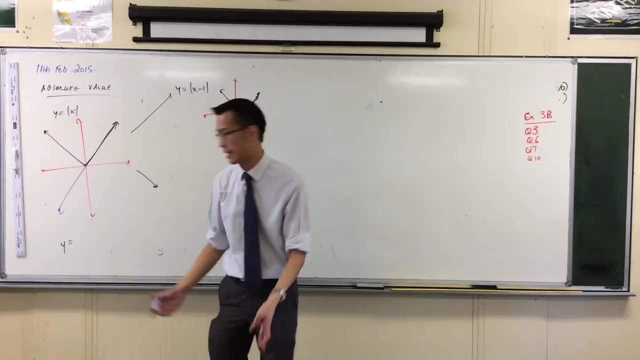 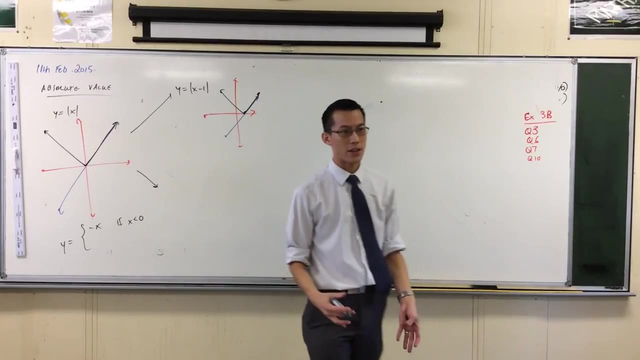 completely differently. they in fact have different equations, and we knew this based on our definition from before. the absolute value of X means two things at two different places: where X is negative, the absolute value of X is negative X, and when X is positive. it's just regular. 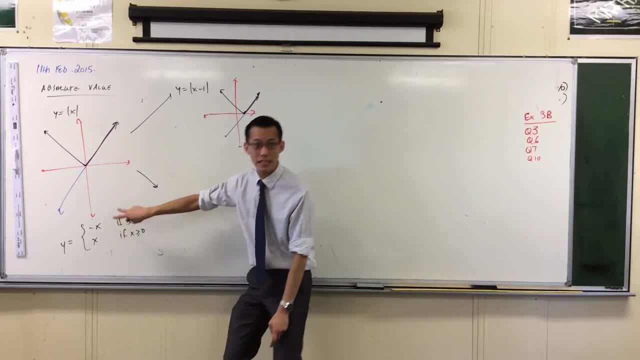 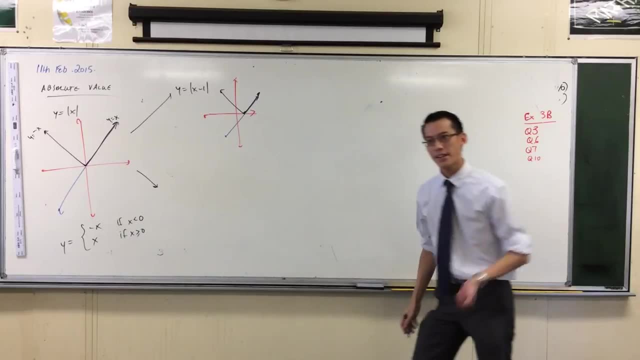 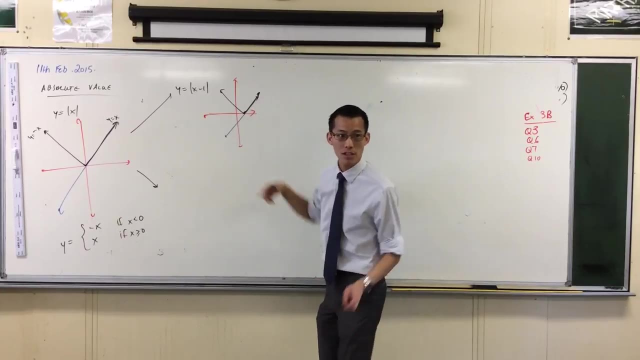 old X. okay, and these two? these two are the equations of my two branches. right, there's minus X and there's X. now, exactly the same way. and you don't need to keep on writing it out in this formal way. you can start to see it right, here's the unmodified part. what's the equation? 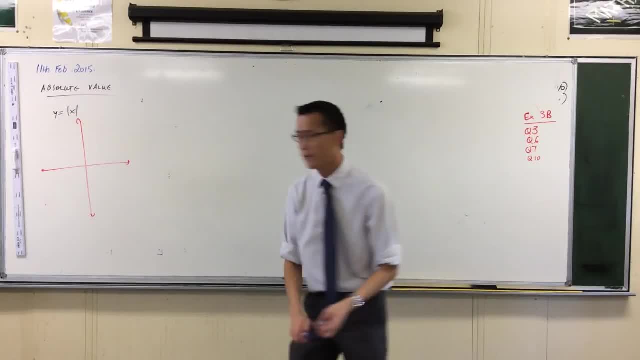 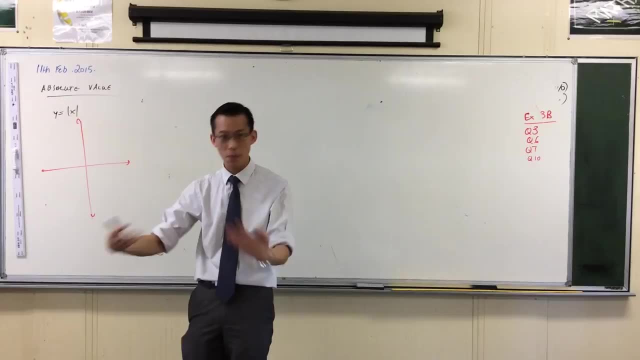 That was the most basic definition I gave you. So therefore, you say: well, this is like y equals x, and I know what that looks like. but you just take the positive values. So here's y equals x. There you go, Good old y equals x. 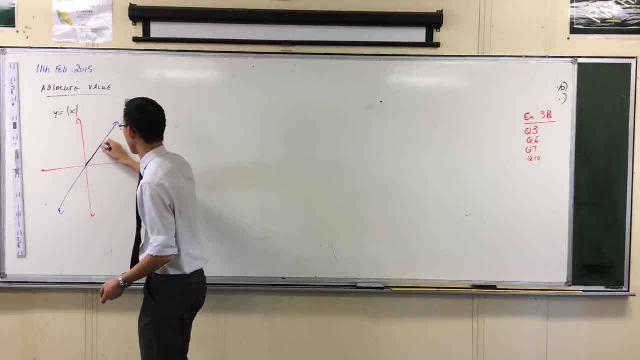 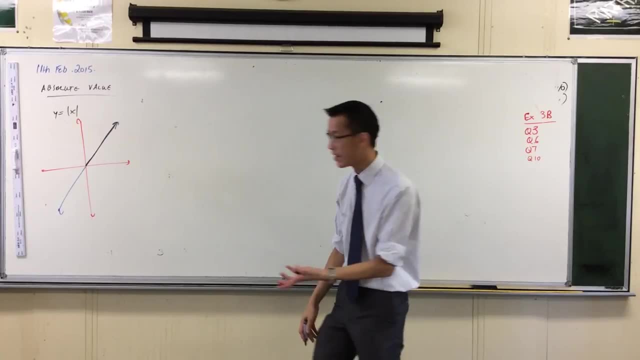 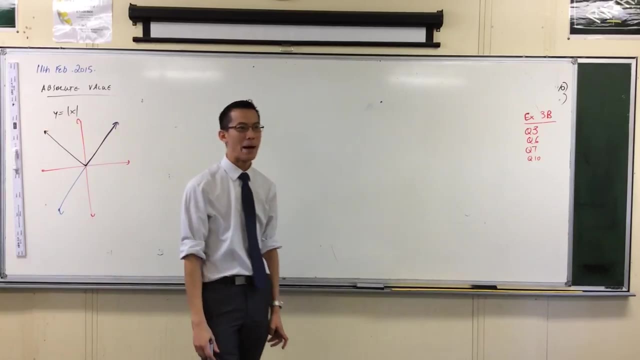 Some of it is positive, so no problems, There you go. That part's all happy times. But on the left hand side I have a whole portion of the graph that is negative, So instead I make that part positive. So most people learn about absolute value graphs as, oh yes, the bouncy things. 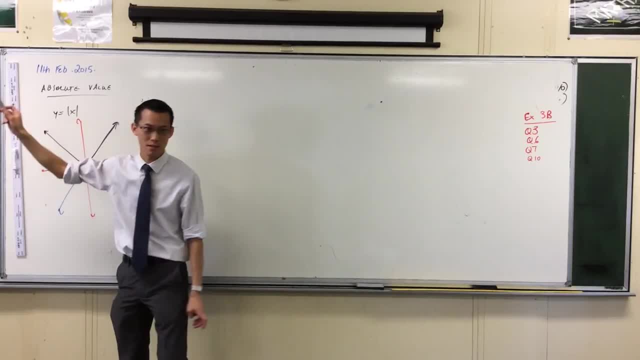 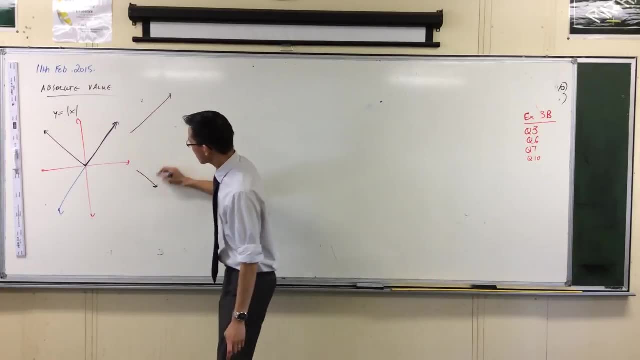 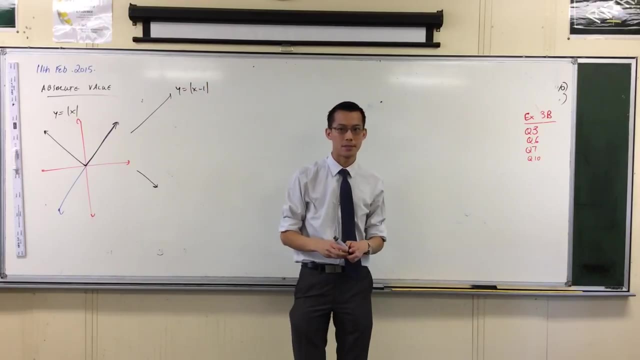 Because they come down to the axis and then they literally bounce. That's not that complicated. Let's think about a couple of variations on this. Let's think about: First, let's modify it within the absolute value sign. so if i said, well, how would this thing be different? okay, so. 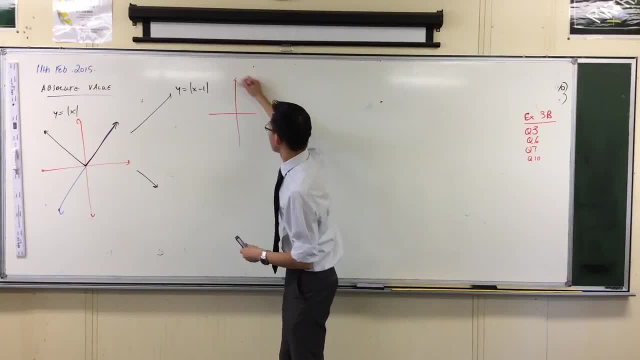 we've looked at this before. briefly again, i'm going to go to this idea of thinking about: what does x minus one look like? okay, and it's just like x, but drop down right and then again i think, well, i just want the positive parts, so this bit's good and this bit is not okay. now this is a really 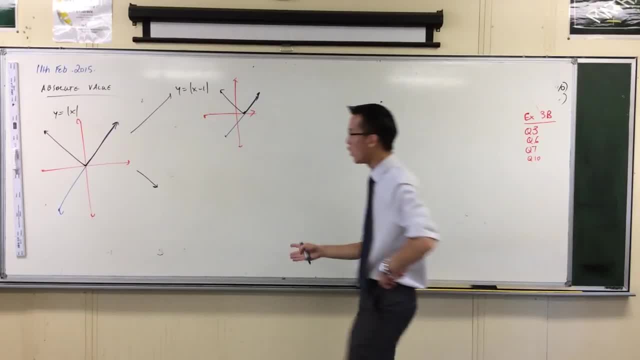 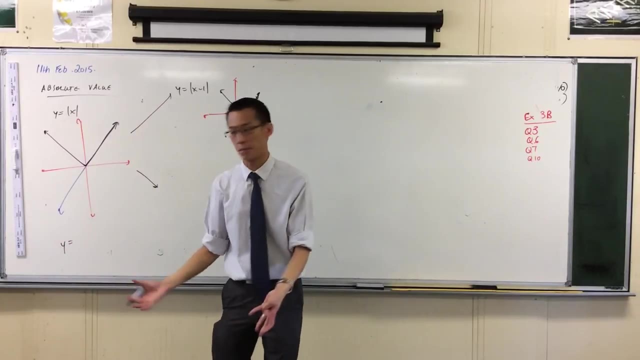 important point under absolute value graphs. i'm going to put this on both of them, because what you've got is two branches that are behaving completely differently. they in fact have different equations, and we knew this based on our definition from before. the absolute value of x means two things at two different places. when x is negative, 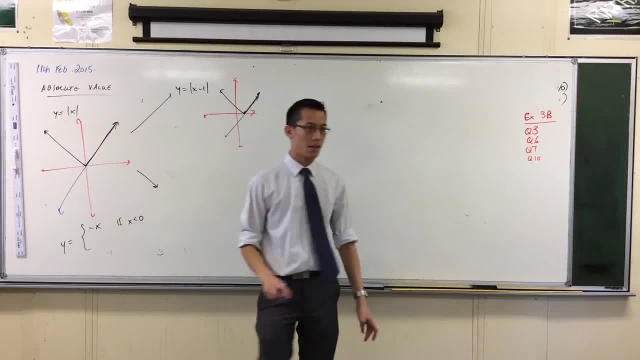 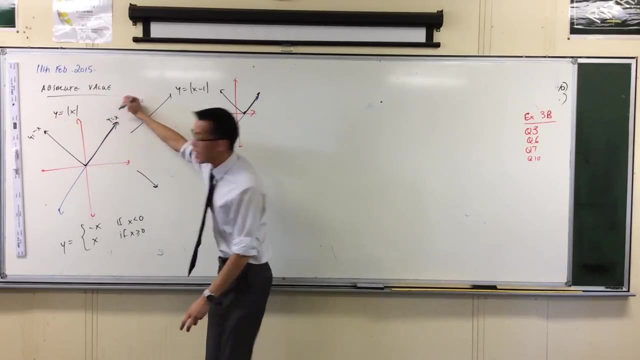 the absolute value of x is negative x, and when x is positive, it's just regular old x. okay, and these two? these two are the equations of my two branches. right, there's minus x and there's x. now, exactly the same way, and you don't need to keep on writing. 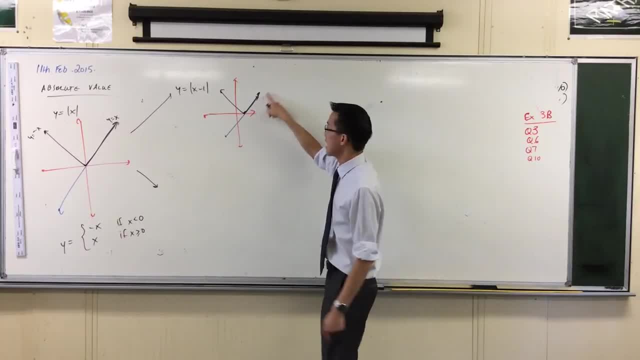 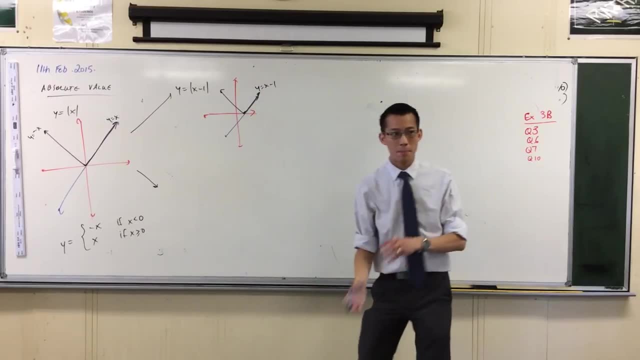 it out in this formal way. you can start to see it right. here's the unmodified part. what's the equation of the unmodified part? it's just x minus one. okay, the part that we've flipped. we've just slapped a minus sign on, right. uh, see there, i've just slapped a minus sign on it. so the effect.